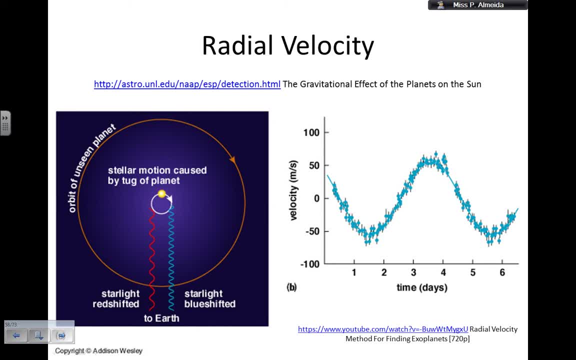 basically what happens is the following when things are moving in relation to you so to towards you or away from you and this this thing is a source of either light or sound any wave there is going to be an apparent shift on the frequency or wavelength or frequency and a wavelength of what that source is sending out so for example imagine that I have a star and that star is moving towards me the wavelengths of that star the certain specific lines are going to shift towards the blue part of the spectrum so we call it blue shift and if the star is moving away from me then the wavelengths of the light are going to go towards and shift throughout towards the red so is red shift so the radial velocity method works by knowing that any objects is going to cause a gravitational pull in another so when I have a planet around 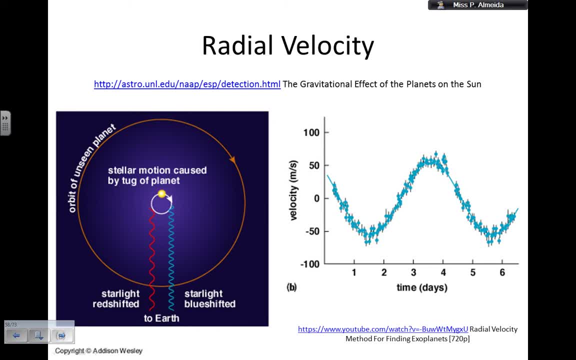 the star the star makes the planet go around around them around it but the planet is going to make the star to wobble around the center of mass of the system so this is the planet going around the star okay and my star due to the gravitational pull to the planet of the planet is going to go around the center of mass of that system as well the planet star system okay so if I'm here on Earth and this system is edge on sometimes the star is going to show blue shift so because the star is moving towards me okay other times as the star keeps going around the center of mass of the system is the star moves away from me so from Earth we get a red shift so what we do is we instead of looking for the planet directly we look at a stars or a star or several stars and we measure the velocity of the stars in relation to us over a certain amount of time and if we get a graph like this one where the velocity sometimes is positive and other times is negative so kind of a sine or cosine wave then it means that the star is wobbling the star is moving towards and away from us in a periodic way or in a periodic motion and the best explanation for this 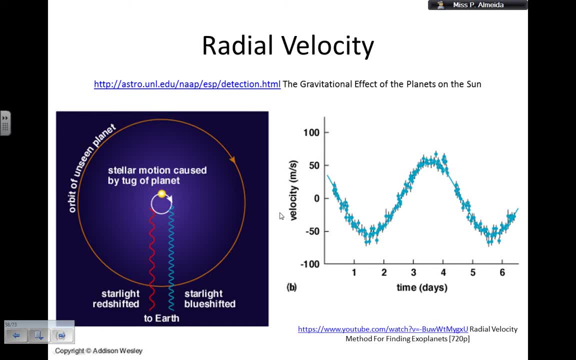 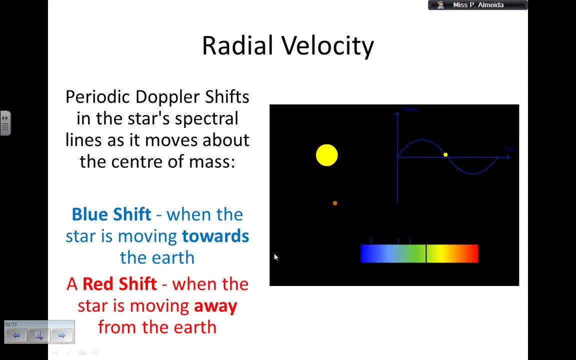 to be happening is that there is a planet around the star okay I'm going to include this link on the description this shows what this is showing in here okay so this is how it works that's the planet right there going around the star okay this makes that the star wobbles around the center of mass of the system which is the planet star so what happens is the star shows that the velocity sometimes increases other times decreases in relation to us and this is how it is if I look at the spectra of the stars which is what I'm going to do okay I see the line sometimes moving towards the red part of the spectrum and other times moving towards the blue part of the spectrum so these three lines here where is where the if the star is not moving where the lines would be and sometimes you see the lines are moving towards the here we go red other times towards the blue okay so that means that my star is going around on the periodic motion and then the time period that this happens tells me the orbital period of the planet okay so I can get a lot of information just by it I can also make an estimate of the mass of the planet as I will show you in a second okay so let 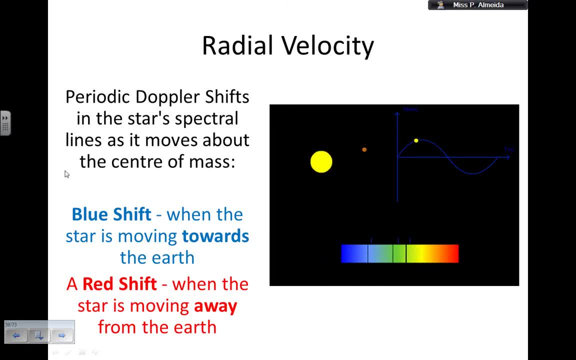 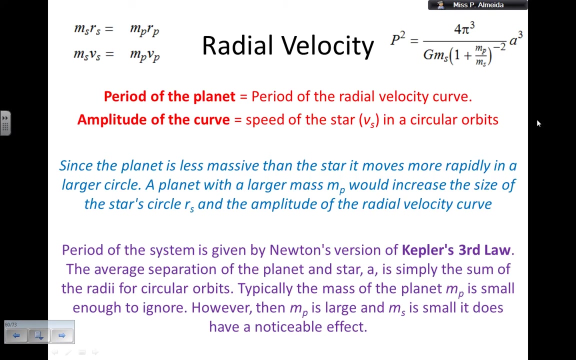 me just before I move on the slide to give you a little bit more information there is a periodic shift in the star spectra lines as it moves about the center of mass and this is because there is a planet around that star that is making it wobble it could mean more than a planet and if it's more than a planet the line doesn't look so pretty as this one but you will be able to identify the different planets okay so I get blue shift when the star is moving towards the earth and red shift when the star is moving away from the earth and as I told you this is periodic and then from the center of mass it moves towards the earth and from the period that it takes for the star to move towards and away from us I can get the orbital period of that planet okay so this is what I can do I can get the period of the planet by using the period of the radial velocity curve okay the amplitude of the curve so how tall the curve goes high and higher up and lower down tells me about the speed of the star in a circular orbit and this gives me information about the speed that the planet is going around the star okay sometimes the line is not very much looking like a sine and or 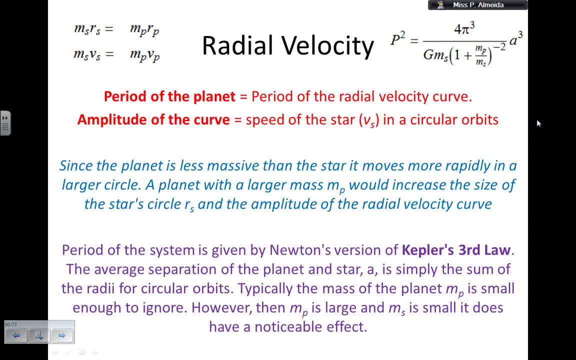 cosine line and is a little bit inclined this gives me information about the planets are eccentricity of the orbit and then I can use these equations the period of the planet squared equals 4 pi cubed to all divided by G the gravitational constant times the mass of the star that multiplies 1 plus the mass of the planet over the mass of the star all of that to the power of minus 2 and I multiply that the whole thing by the cube of the semi-major axis okay and here is how the relationship works the mass of the star times the velocity of the star equals the mass of the planet times the velocity of the planet I can do the same for the radii okay so you don't have if you're doing this at a level because you're taking the astrophysics option you don't need to know these formulas into this detail you just need to have an idea of how the radial velocity method works in finding out the planets okay so the planet is less massive than the star and it moves more rapidly in a larger circle okay so the planet with a larger mass would 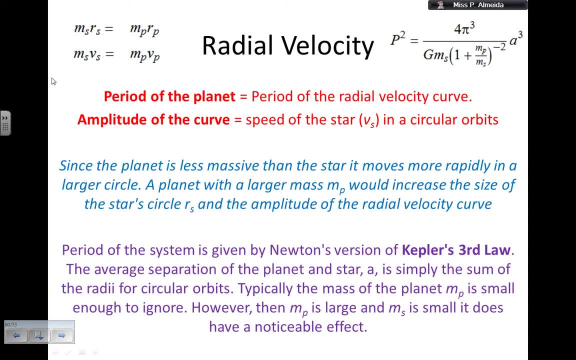 increase the size of the star's circle and the amplitude of the radial velocity curve okay and then if I want to get the period of the system I get by Newton's version of the Kepler's third law which is this one here on the top okay so that's the Newton's version the average separation of the planet in the star and this they have that average separation is a is simply the sum of the radii for the circular orbits typically the mass of the planet MP is small enough to ignore so you can take it away in your calculations however when MP is large and MS is small it does have a noticeable effect now this technique is biased towards a certain specific type of planets this radial velocity technique is biased towards larger mass planets because the larger the mass of the planet then the more is going to attract the star to to move away from a center of mass of the system so the more the star wobbles so I get the curve to be more notes notables also the period of the orbit is also biased towards planets they are